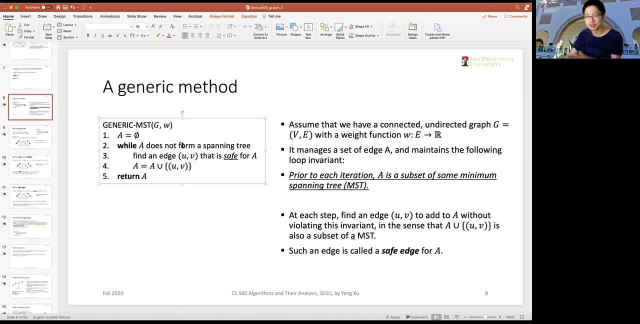 edges to the empty sets incrementally, Like in each. within each iteration of the while loop, you will need to select an edge from the remaining, from the from the graph that is outside the set, And that edge should be should satisfy some criteria so that it is safe. Okay, So the after. 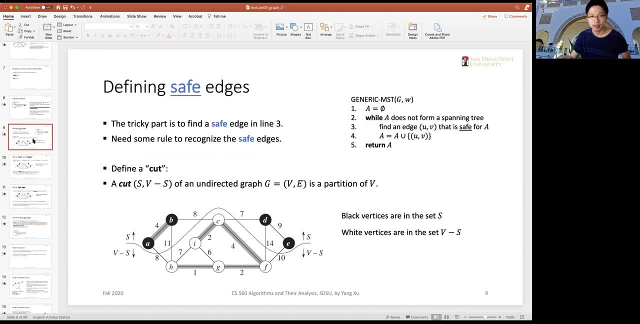 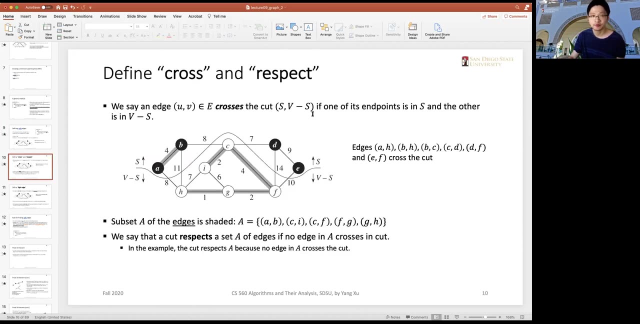 we defined the generic methods. we actually introduced a bunch of terms like the cut of a graph which splits all the vertices into two partitions And the term for cross right. So if a, an edge is the two ends of the edge exists in the two. 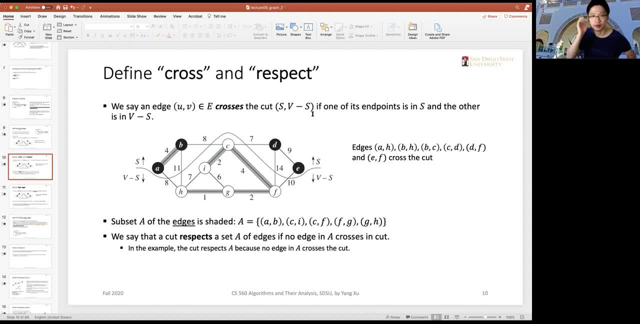 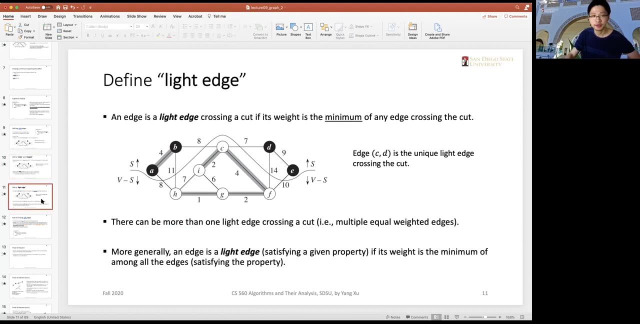 in the remaining, in the resulting two partitions of a of a cut, then we say that edge crosses the cut. And also we say a cut can respect a set if there's no edges in the set that crosses the cuts. So we use this bunch of definitions to 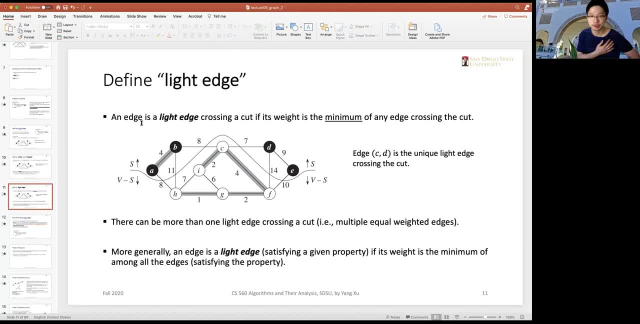 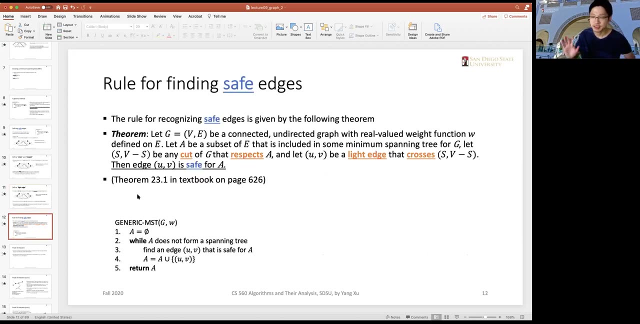 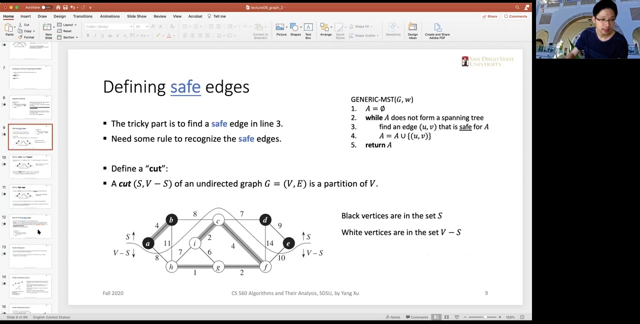 define the light edge, which is the least weight, the edge that has the minimal weights among all the edges that cross the cuts. So we say that a light edge is some is a safe edge. Okay, So the this slide- from from slide nine to slide 12, we basically lay out a very 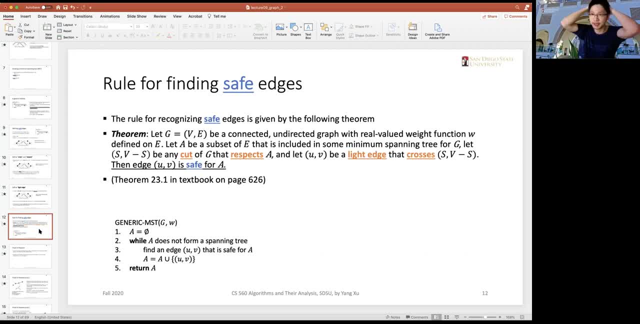 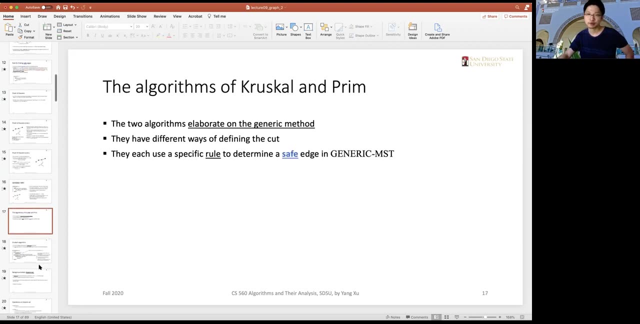 high level principle of selecting a safe edge And based on this principle, we can have the two implementations, which is Kruskal and the Prim's. So the plan for today is that we cover the Prim's algorithm. So basically, Kruskal's algorithm and the Prim's algorithm. they use two different. 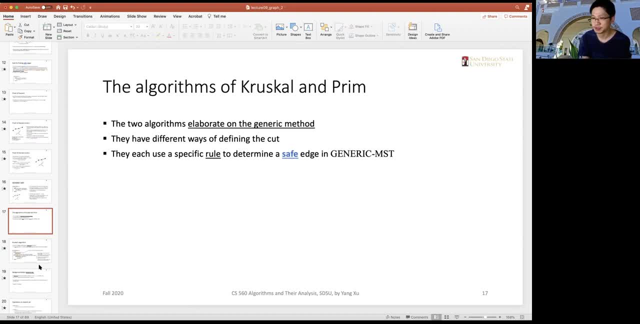 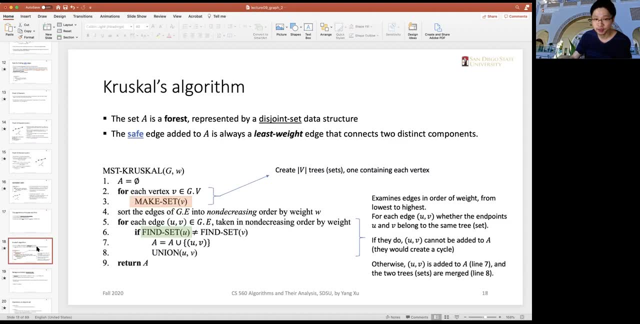 ways to selecting the safe edge. And let's review Kruskal a bit. So the Kruskal algorithm relies on the disjoint set. Okay, so the disjoint set supports several primitive operations like initialize a set from a vertex, which is done by calling the make set, And also to find: 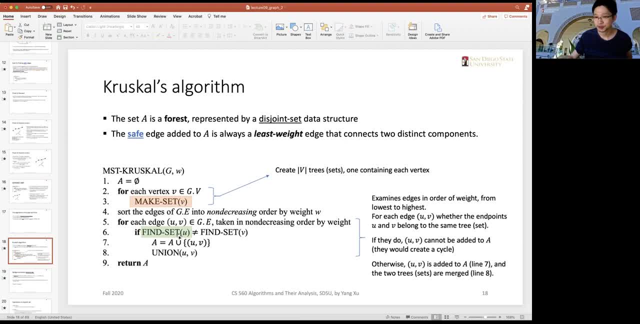 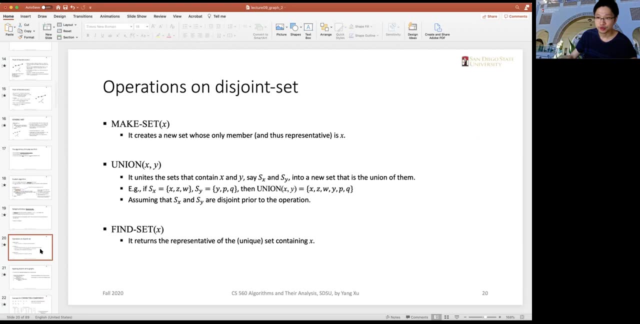 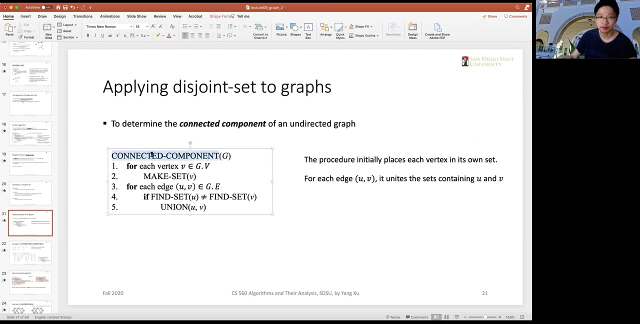 the set- that's a vertex that belongs to- by calling the procedure find set And also union, which merges two sets. So, given this disjoint set data structure, we're able to define this connected component procedure. So this procedure will help you find all the connected components within the graph. Okay, so the assumption for running. 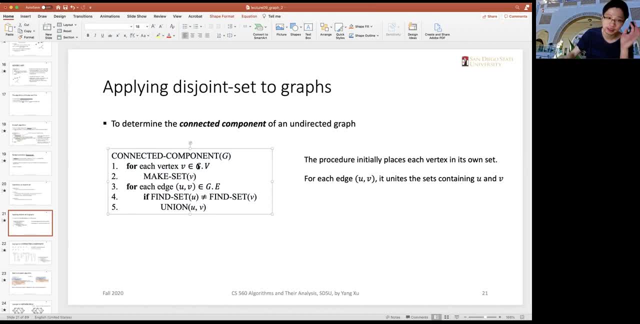 for running this connected components graph, connected components algorithm procedure is that we don't assume that all the vertices are connected in a graph, So that's why we want this procedure to find all the connected components. Okay so, and we will later apply this connected component procedure to the cross-codes algorithm, but the 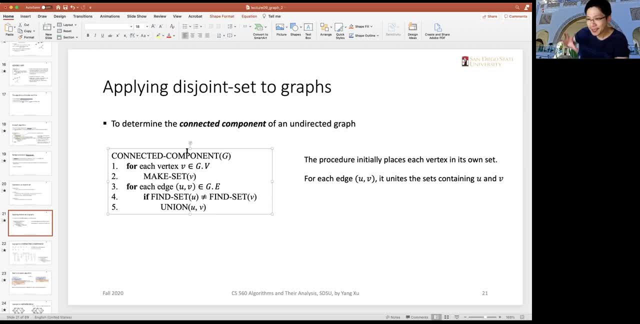 assumption of a cross-codes algorithm is stronger because cross-codes algorithm is to solve the minimum spanning tree and this assumption of the minimum spanning tree problem, that is, that we are able to reach all vertices in the graph and they are all connected, otherwise it won't be a spanning tree. 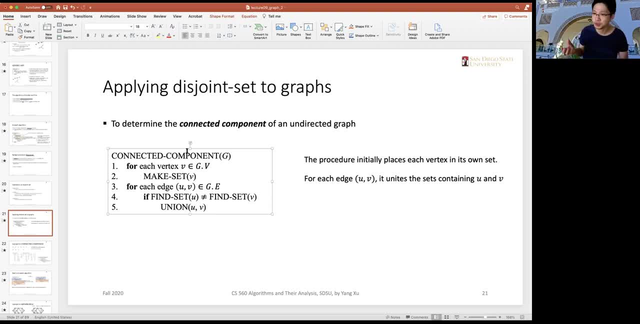 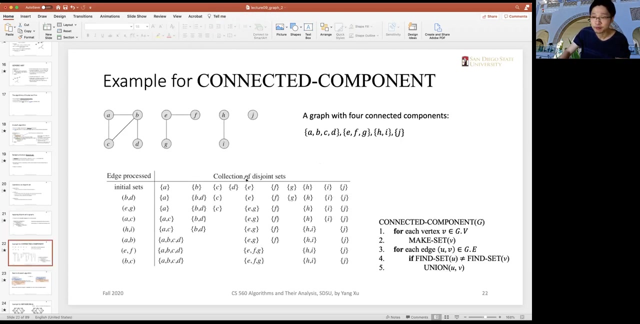 right if, if there are some vertices that are not reachable from the source, then it's it's. it's violates our assumption at the beginning. okay, so, roughly speaking, the connected component defined here is a more general, a more general method and through running, by running this example on the demo here: 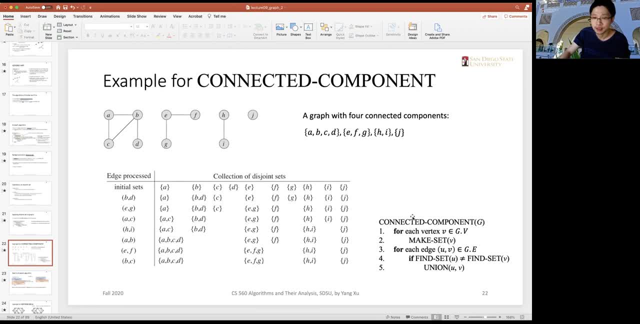 we're able to see the. that's how these connected components. algorithm merges distinct joints together. as long as there's some, there's no edges. if if there's, if there's edges that connect to component to connect to vertices, then the algorithm is able to make is to union the two vertices together. 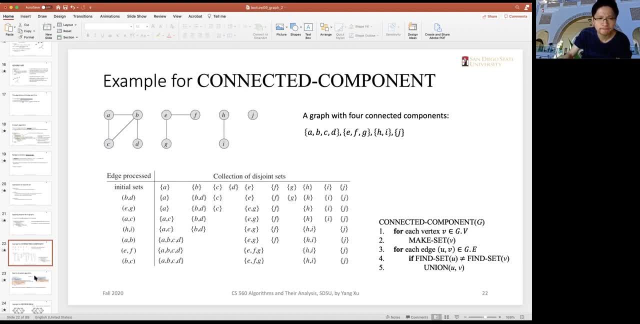 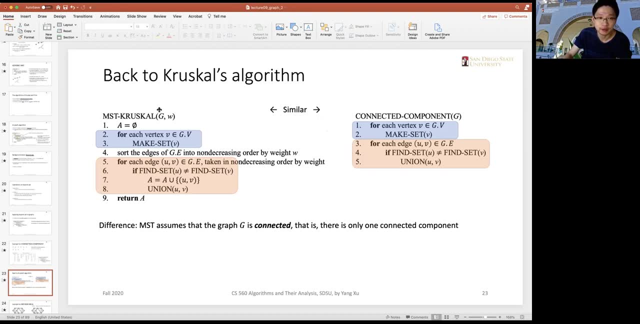 so the what's difference between the what's different between the cross-codes algorithm and connected components algorithm we listed. by comparing the code, we can find a very significant difference, which is which lies at the line 4 right. we basically need to first sort all the edges by their weights. yeah, 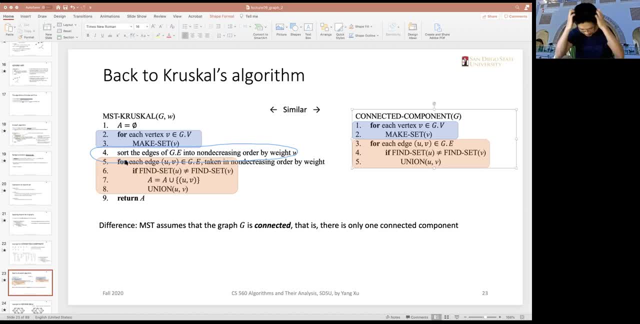 so because that is determined by the, by the, by the nature of the problem, right, we, we, we want to select a. we want to select a, a safe edge and, according to our conclusion from the general, from the generic mst pro algorithm, and safe edge is a light edge, right. 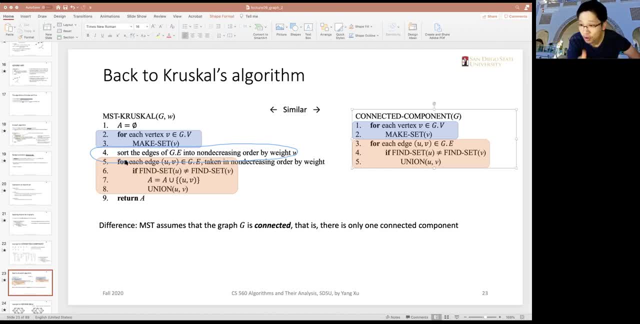 and what is a light edge? light edge is among all the edges that cross the cut. it must have the minimal weight. so that's why we- it makes sense to to first sort all the weights, sort all the edges by their weight, so in the after we sort them in the next uh, in the uh, in the 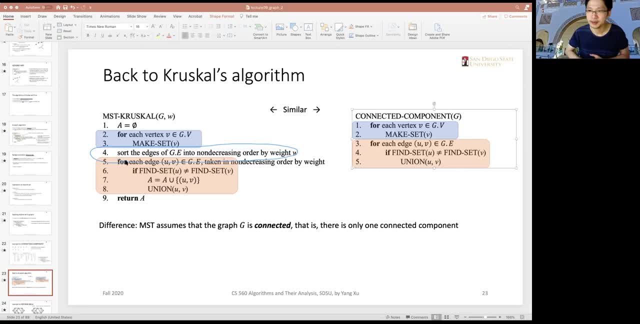 next for loop, we're able to iterate over, uh, all the edges in the desired order, right? so, um, everything else other than the sorting part. everything else other than the sorting part, it's basically uh, the same thing, uh, that occurred in the connected components algorithm here. so an additional step is that we need to put the edges selected into. 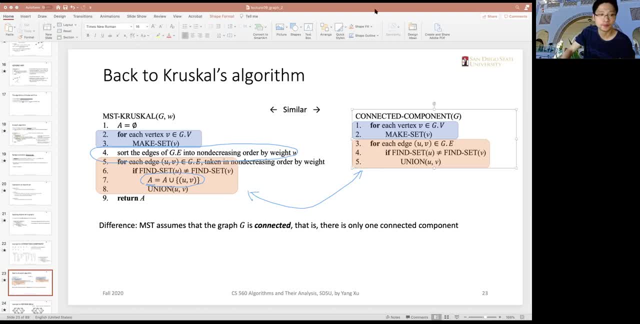 into the empty, into the set a. okay, so. so we can kind of conclude that the way that the cut uh and uh that, or the way uh that the safe edge is selected in classical algorithm is to uh, to look at the weight of the edge right and as long as that edge uh connects two distinct 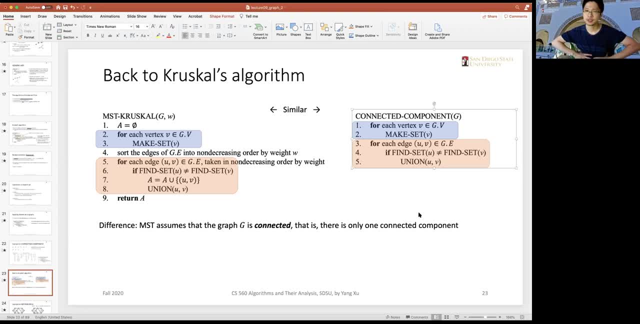 joints and also it is uh currently the smallest uh, uh, the, the minimal the weights. that has the minimal uh the edge with minimal weight. then we can connect, consider it for the safe edge. And another characteristic is that all the vertices are initialized to the, initialized to the sets. 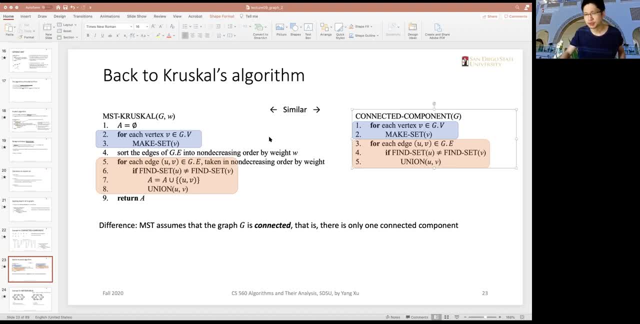 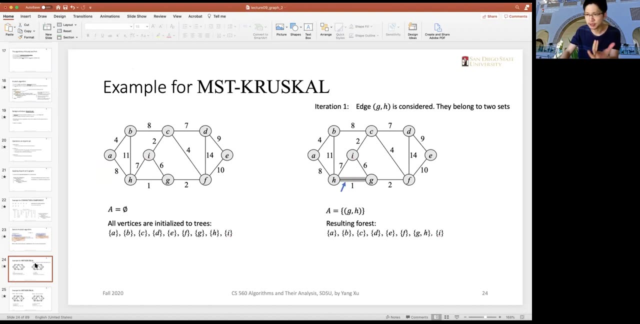 So we can think of that. all the edges and the vertices they form. they form all the edges in the selected in the set A. they form a forest, because it's not for sure that's after each time we select a safe edge. they must form a tree. 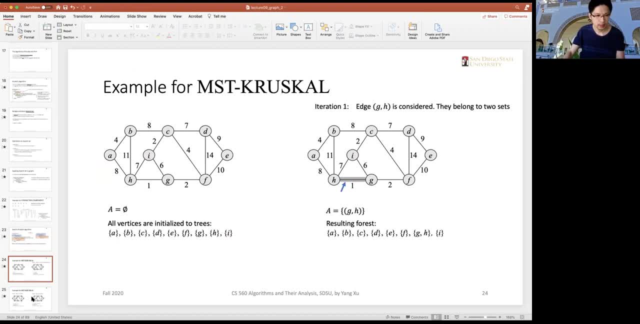 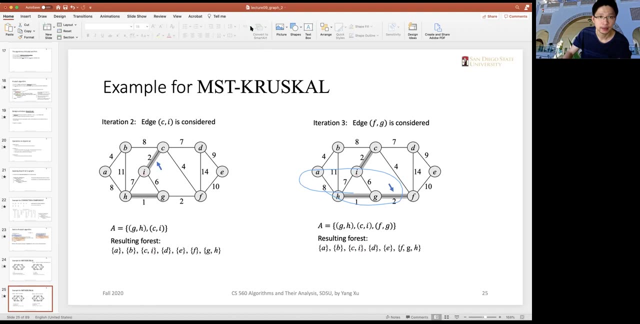 It is not the case. So, for example, here: yeah, after step one, after step two, here, after HG is selected, then the next one to be selected is IC. okay, Because it has the at least a weight right. 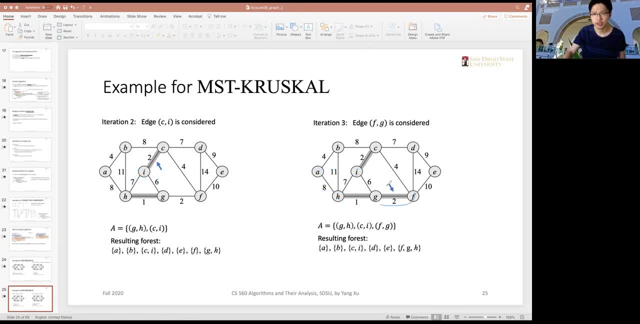 And then the next step is GF. So it's not necessarily true that what's inside A is always a tree. It's, but rather it is a collection of trees. So it is a forest, And only after all these steps are done. 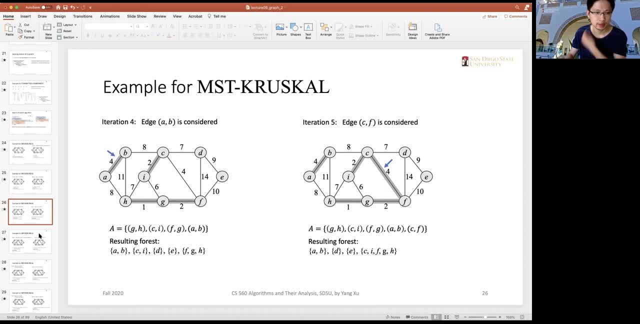 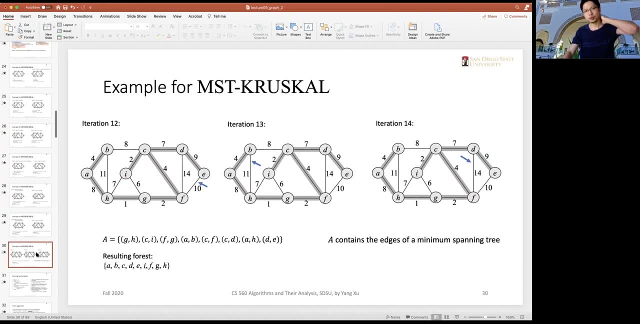 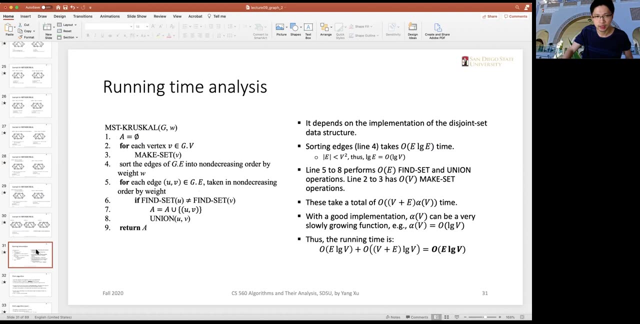 we will have a complete tree. So in any intermediate steps we can have multiple trees in the set A. okay, So this is a very salient characteristic of the cross-codes algorithm And we today we're going to see the PREEMS algorithm. 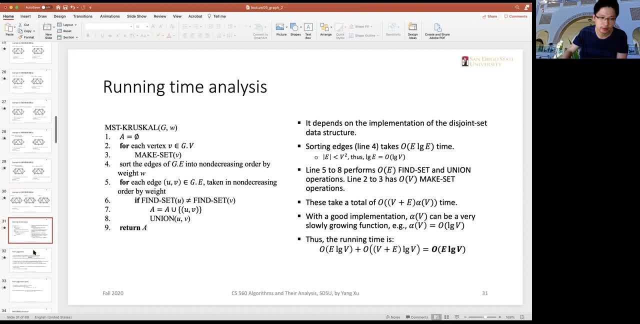 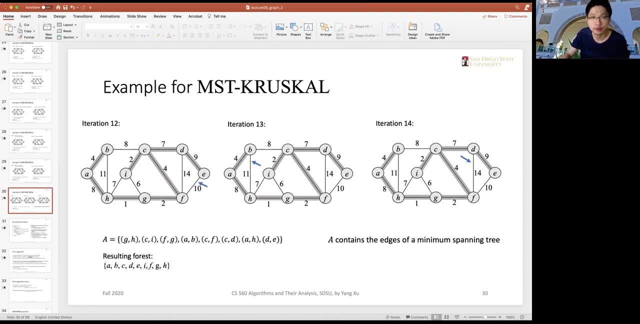 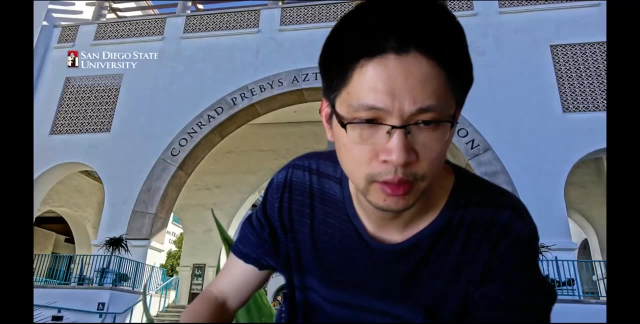 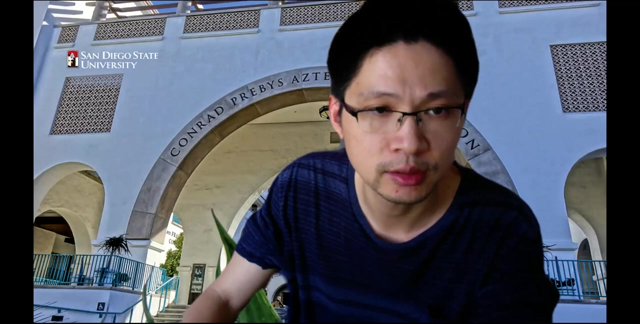 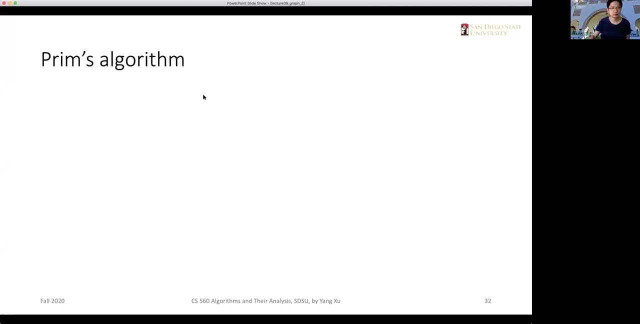 will be different from the cross-code in terms of the way that the tree is constructed, So let me switch to the playing mode. Stop sharing and start playing mode. Play the slides and share the screen again. Okay, Hello, hello, Hello, welcome to my presentation. 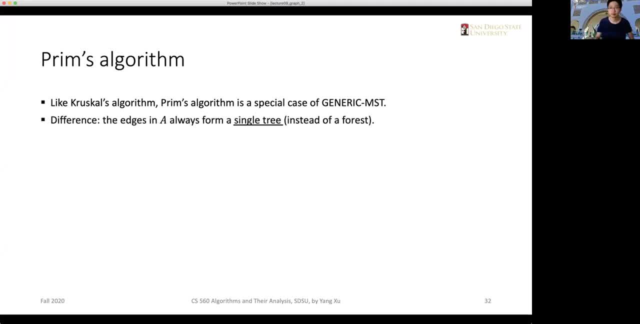 This is a presentation of the PREEMS algorithm And it's just another special case of the generic MST. okay, We actually implemented the algorithm based on the same thoughts And the difference is that all the edges in A always form a single tree. 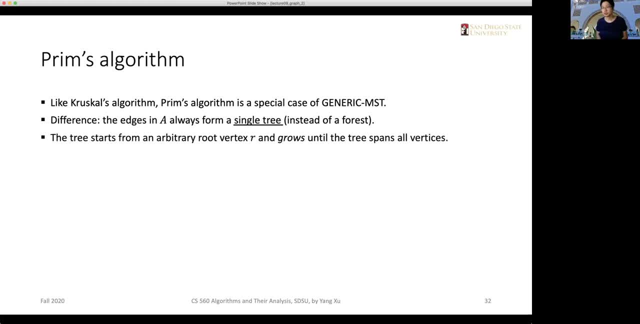 not a forest, like like cross-codes algorithm, does start from an arbitrary root vertex. R. A tree always grow from a root node, from a root vertex, And we will grow the tree until all the vertices are spanned, until the tree spans across all the vertices. okay. 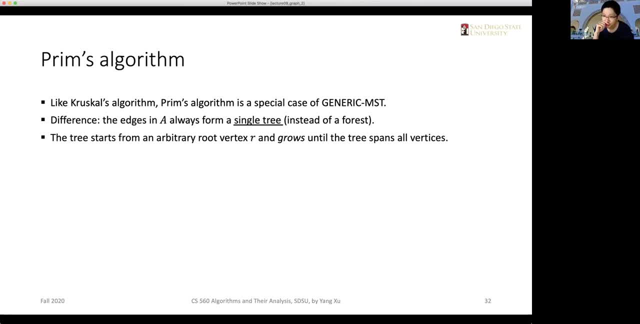 So now we'll need to use a second, a new data structure, right? So it's different from the disjoint data sets that we used in Kruskal, And this time we'll need to use a minimal priority queue. So this is a familiar name, right? 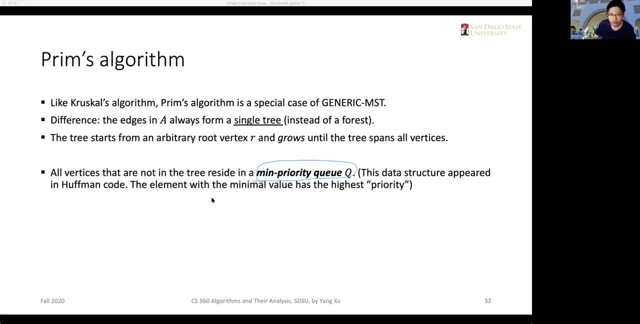 The minimal priority queue will be used to store all the vertices that are not yet in the tree. okay, So in the Huffman codes we use minimal priority queue to store all the letters with their frequencies, right? So the minimal priority queue is a queue structure. 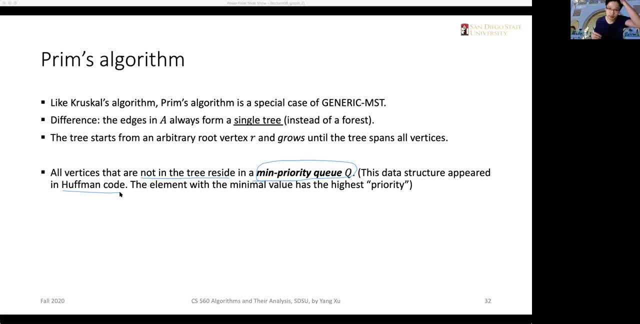 Basically it's a first in, first out data structure, but the priority is measured by a score and the elements with the minimal score values, with the minimal values, will have the highest priority. That means the vertices that has the minimal score values will be extracted first. 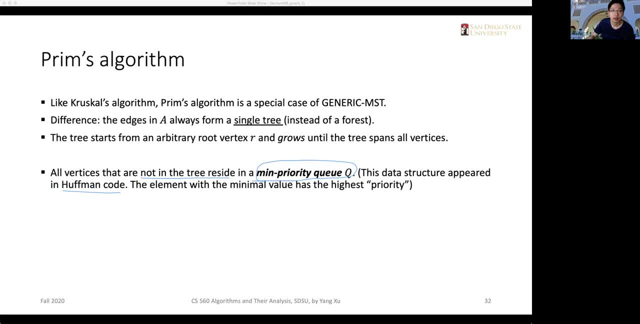 will get out of the queue. first Let me open up the chat. So it's a basically a queue like structure, but with the priority scores with this specific way. So we need to use a queue. you need to use a key attributes for each element in the queue. 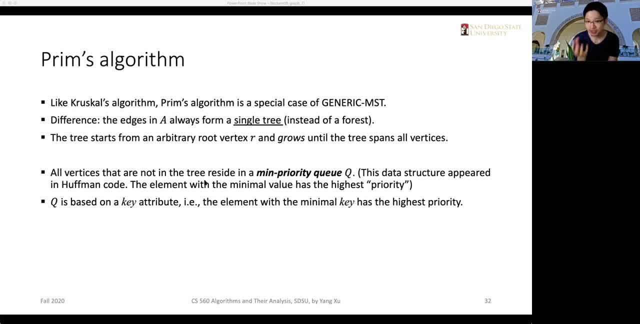 Okay, So the elements with the minimal key will have the highest priority. So this is some infrastructure we need to use The queue and all the elements in the queue will have a key attribute. okay, And for each vertex, the key is defined by the minimal weights. 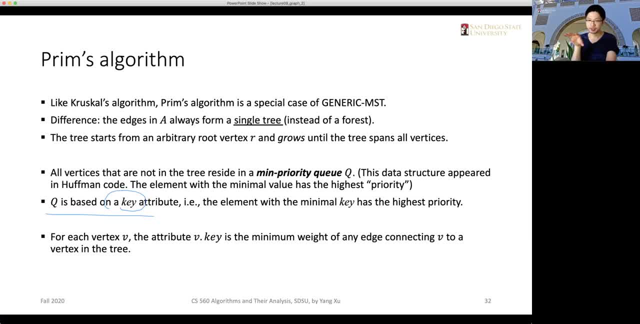 of any edge that connects the current set, The current vertex V, to a vertex in the tree. Okay, So if there is an edge that connects the current vertex V to a tree, there could be multiple edges right To a tree. There could be multiple edges to the outside vertex. 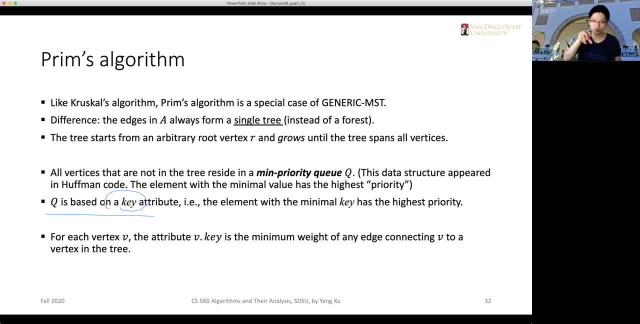 to the current tree, But we need to choose the minimum weights as the key value Right, Because remember the principle of finding the safe edge, and the safe edge needs to be the light edge, And light edge is the one that has the minimal weights. 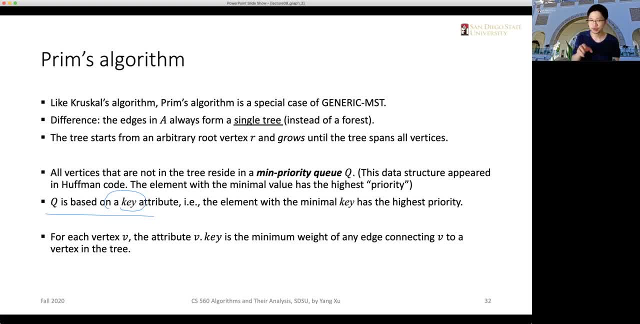 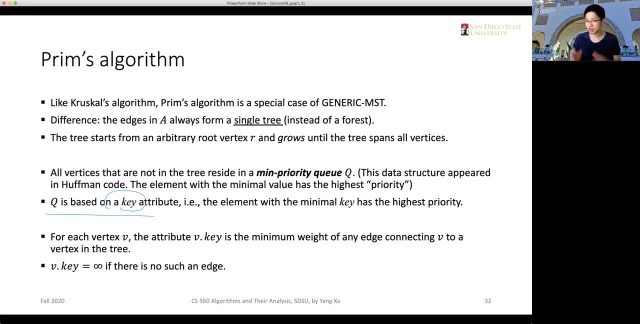 Give it an infinite number to indicate that, okay, this current is not connected to the tree yet, So we will not consider it. consider it in this round, Right, But it once, but after a while. we are growing the tree. 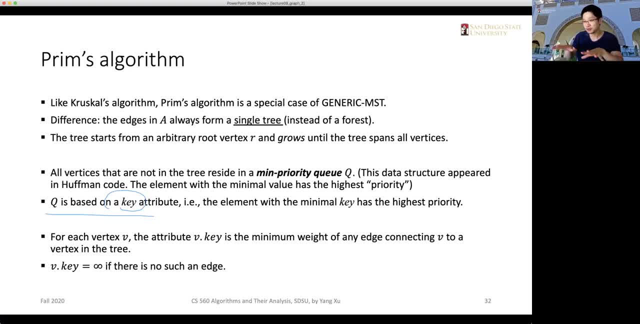 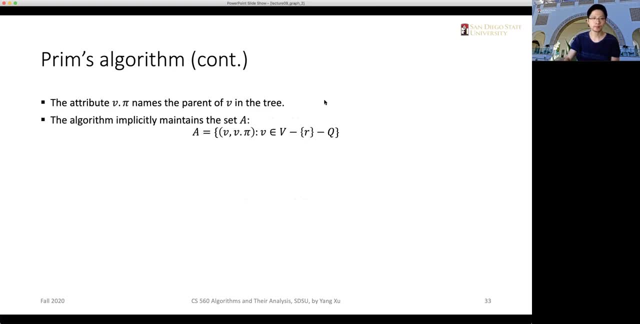 the tree is getting larger and the spanning to larger areas in the graph, then more and more vertices will be likely to be will become connected to the tree. All right, So let's look at the algorithm. Okay, So let's look at another: other conditions. 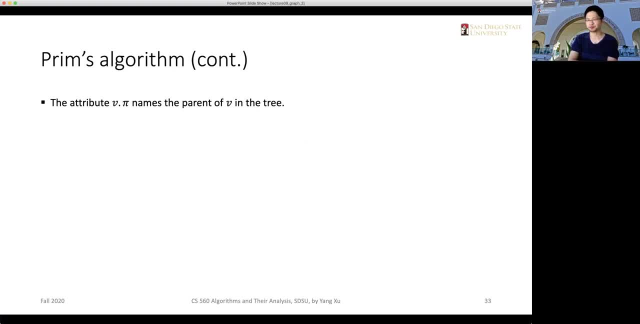 Other than the key attributes, we will also use the use, the parents, the PI attribute, to remember the parents of the vertex in the tree, because now we are growing a tree rather than disjoint, rather than using disjoint sets, So we'll need to use the parents of attributes. 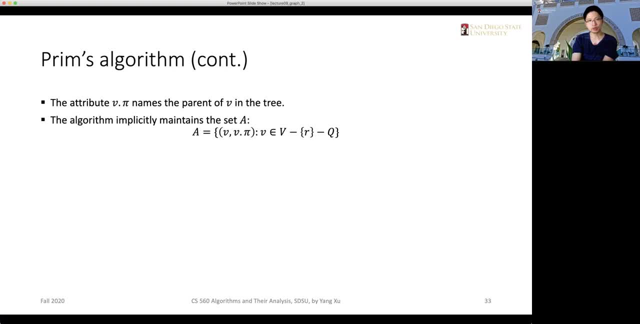 Okay, So these it's, although the all the edges and the vertices are stored in the tree and eventually it is the tree object that we return, but it's implicitly maintained, a set So for taking any key, any vertex in the tree. 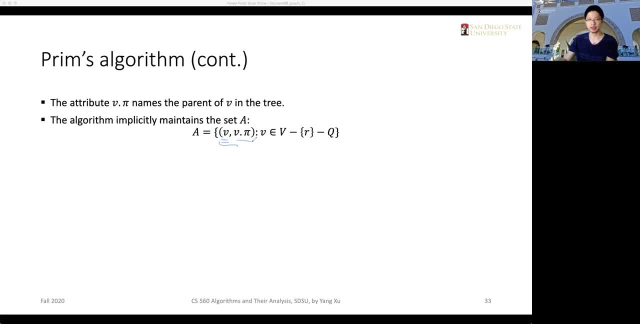 we just use V to its parents to indicate a, an edge right. That is an edge From V to V's parents. that is an edge, And the V is from these sets, and these sets means that V is all, the, all the vertices. 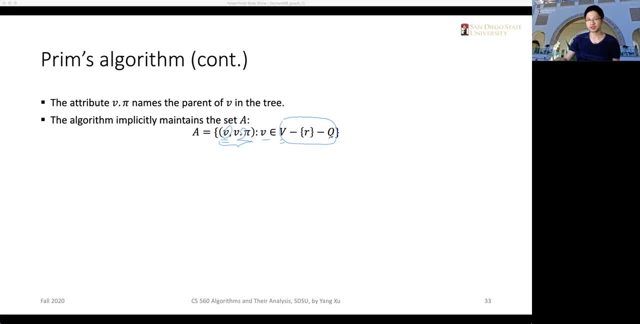 We exclude the vertex in the roots. We exclude a vertex roots And we also exclude the all the edges, all the vertices in the queue, because the queues are are those not in the tree yet. So what's in the tree's actually can be represented by this. 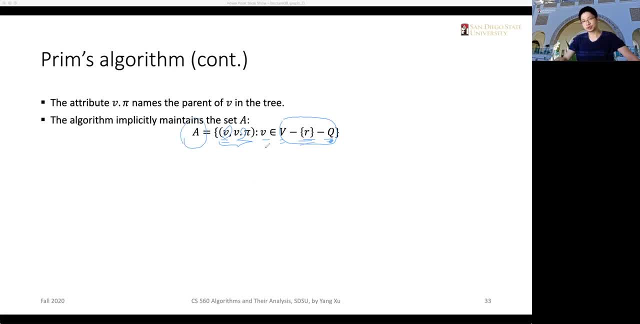 sets. so we exclude the roots, because the roots doesn't have any parent node yet. so that's just for the validity of the definition. okay, so that's the how we define the set a. so when the algorithm terminates, the q becomes empty and the whole set of a becomes this thing. 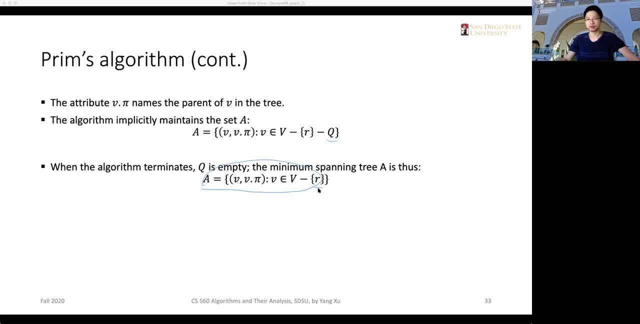 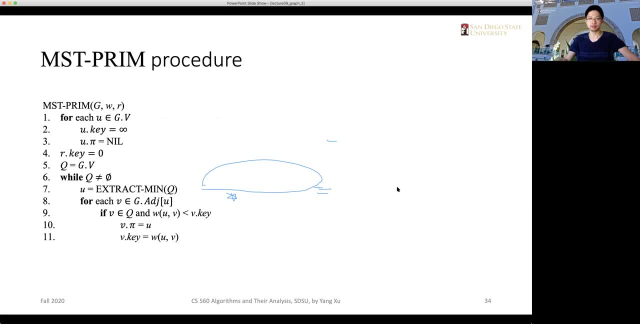 then the only thing that's different is that there's no q here, because q is empty, and at this step we'll simply return the a, and this is exactly the minimal spanning tree we need. okay, now let's look at the algorithm. all right, so this is the mst prims algorithm. 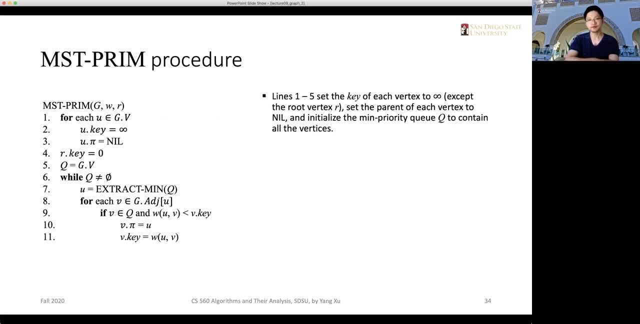 um, first of all, initialization: from line one to line five, we go through all the vertices in the graph. okay, so we're going to go through all the vertices in the graph, except for the roots. so we will set the key to infinity and all the parent to uh, nil, which is for none. okay, and then 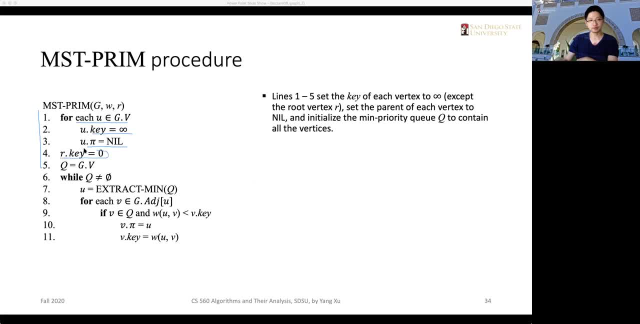 except for the vertex, for the root vertex, because the roots needs to be included in the tree. so we will set the key to be zero, okay, and that indicates it's zero distance away. it's zero, uh, the. the distance from the roots is zero from the tree itself. so, and then, after the initialization, 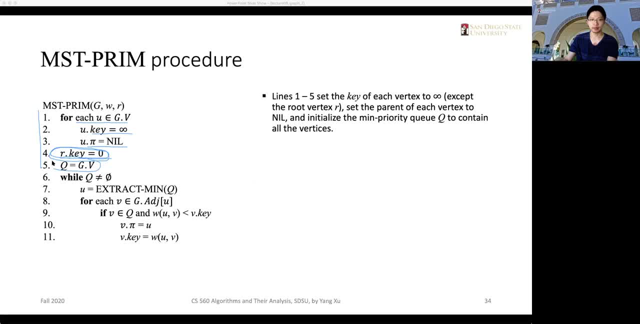 we will initialize the minimal priority q by putting all the vertices into the q first. okay, we will insert all the vertices to the cube, including the including the- the root vertex right, but since the root vertex has the smallest key, so it will be the first one being popped out. 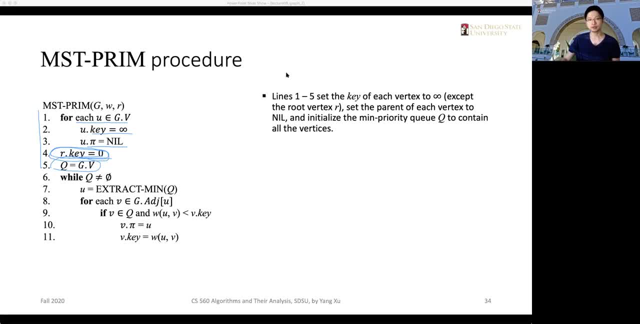 from the queue. okay, so that's it for the q. so let's go ahead and look at the next step: initialization. then in the main body, from line 6 to line 11, we can spot two loops: right, it's a bigger outside loop is a while loop. okay, so it keeps the looping until the the queue is empty. 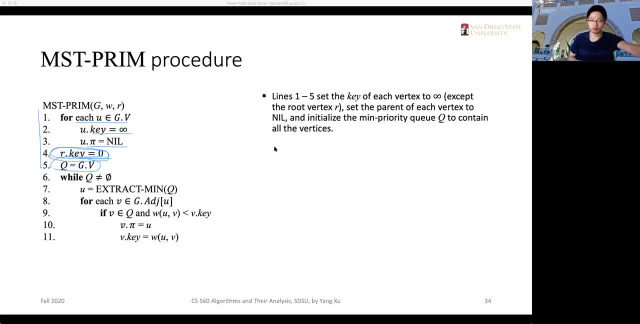 right, as long as there is elements in the queue, we will continue around the code from line 7 to line 11. so in line 7, okay, so yeah, after. let's look at these two bullets again, oops. so before the line 7. after initialization: all the vertices in the queue: if there's any vertex. 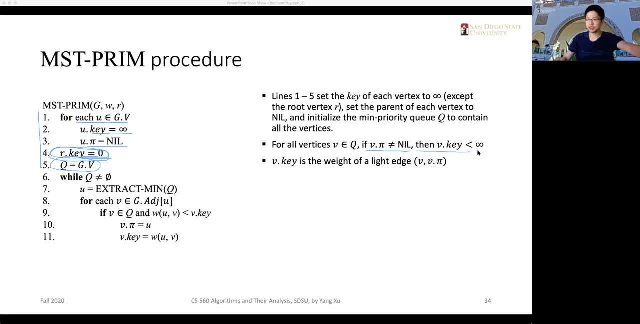 whose parent is not now, then its key will be also be a, an actual number, a valid number rather than the infinity, and and the key is the key attribute that we define first, and it is the, actually the weight of the light edge from v to the parent of v. okay, so let's look at line 7. so for line 7, we 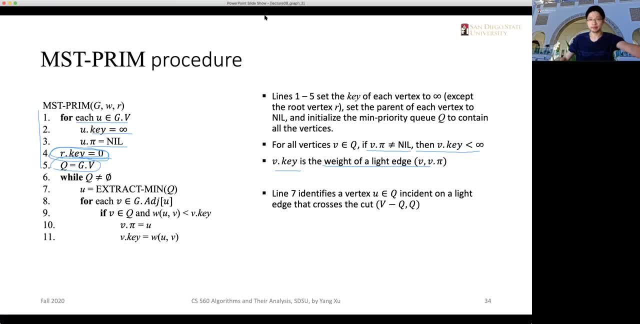 define the vertex as a, the minimal uh, the, the elements, that with the minimal priority, that with the minimal key uh values. okay, so we'll call this extract minimal uh function on the queue. so it actually serves as a function of to identify the vertex uh on the light edge that crosses the cuts. 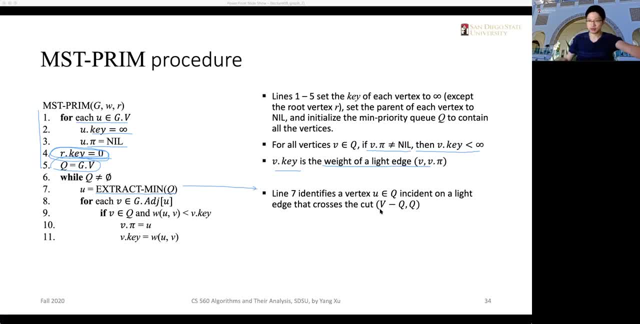 okay, so the cut is defined by: uh, what's in the, what's in the tree? okay, what's in the tree and what's outside the tree. so everything outside the tree is in q and we will remove the u from the queue. pop it out from the from the minimal priority. 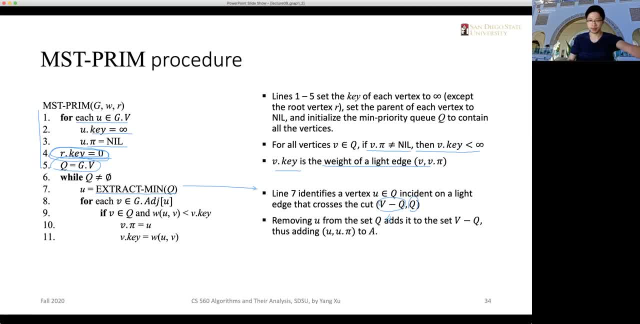 queue and then insert it into the set okay, which is to add the current uh, which is the currents uh insert to the, the edge to the queue from you to use parents, okay. so another important step after we extract the uh, extract the minimal elements from the queue, is 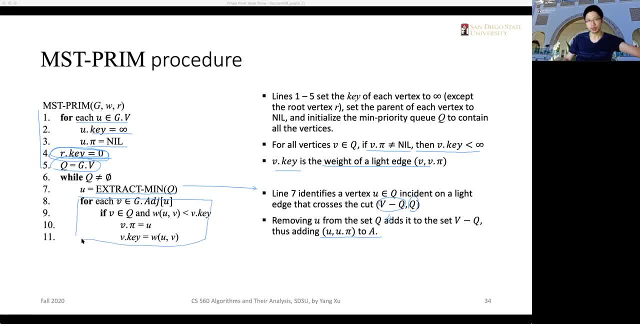 line 8 to line 11, which is a full loop, and in this for loop we actually go through all the adjacent vertices of the elements. that's just. which is u After u is extracted from the queue, we will go through all of its adjacent vertices. 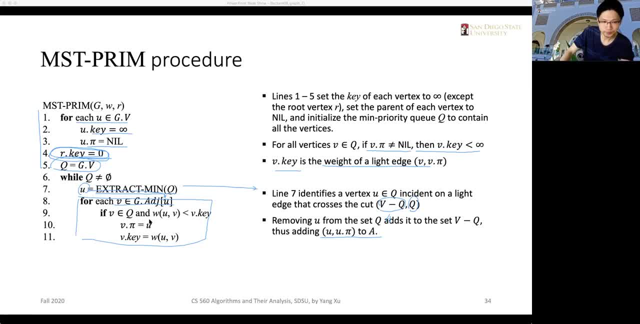 And what we do is to first check whether the adjacent vertex is in queue. If so, we also need to check whether the weight from u to that adjacent vertex is smaller than the current key attribute of the adjacent vertex. If the weight is smaller than the key value, then we need to update the key values for v. 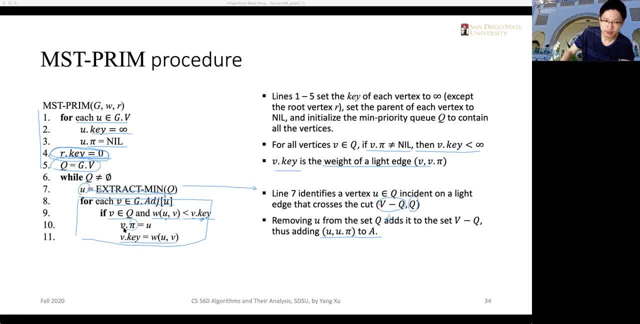 and also update the parents of the adjacent to u. So this may be not that easy to connect at this point, but we'll later see in an example that why this is the case. Because if the weight is smaller than the current key, which means that we find a shorter path, 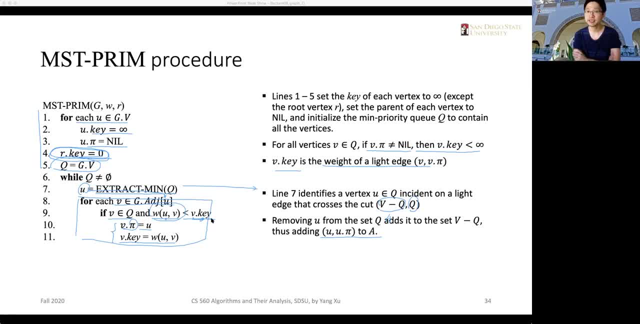 or we find a new light edge to replace the old key values. So it updates the key and the pi attributes for every vertex that is adjacent. But v is not in the tree yet. It must be in the queue. If it's not in the queue, which means it's already in the tree. 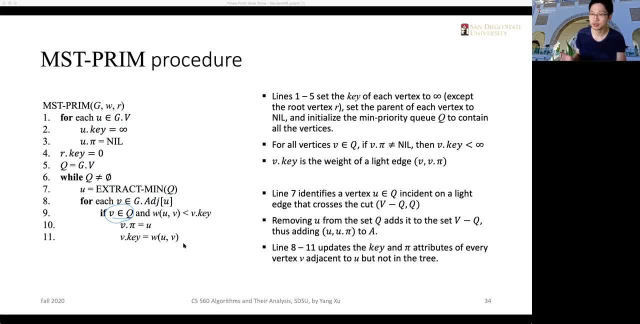 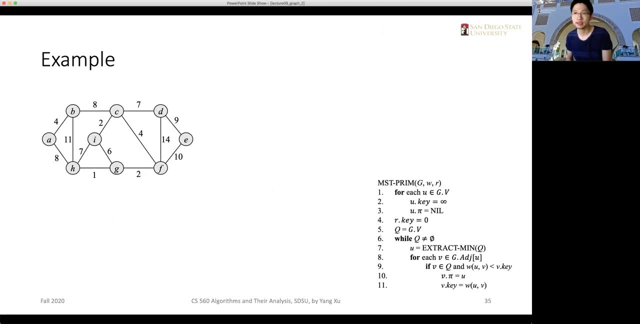 then we don't need to check, We don't need to update it, Because it's already in our minimum spanning tree. We only update those adjacent vertices that are outside the tree, that are in the minimum priority queue. So let's use an example to see how this works. 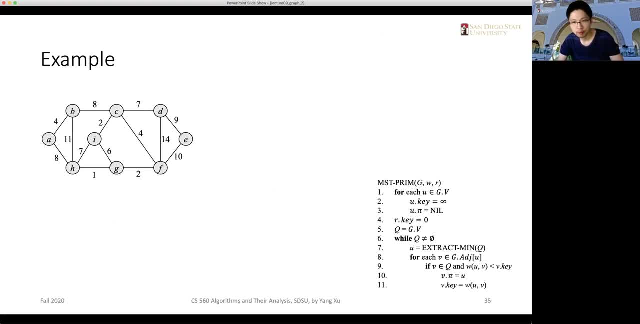 I think this is the same example And we'll run the MST Prim's algorithm on it And we assume that we start from the vertex a, So a will be the root vertex in the tree. So it's highlighted with bold here, So its key value is initialized to zero. 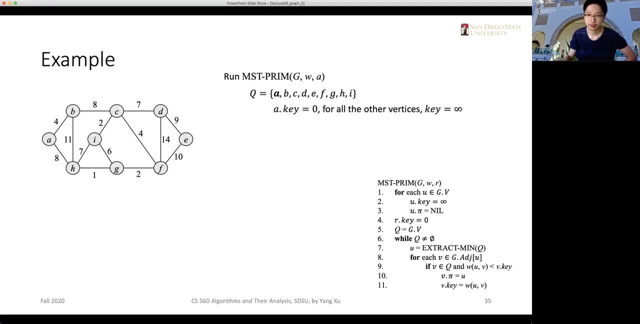 And meanwhile for all the other vertices they are initialized to infinity. So we'll use a queue, We use a table to represent the minimum priority queue. So initially all the elements are in the queue right: A, from a to i. 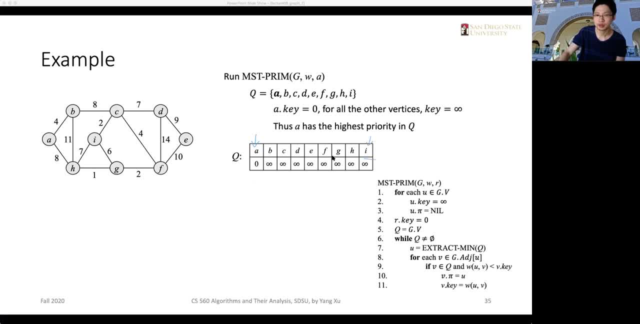 And we also include the second row. The first row is the, So this row is the key values. okay, We listed all the key values here, So, other than the a, all the other elements than a have the infinity as the key values. 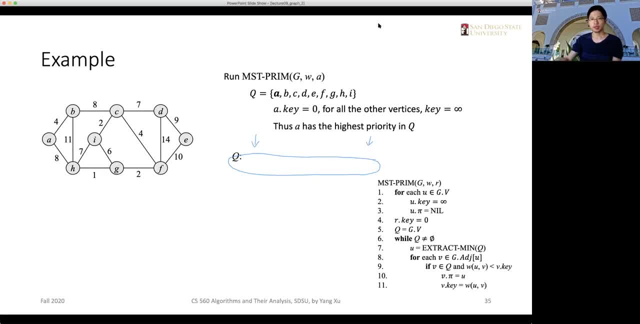 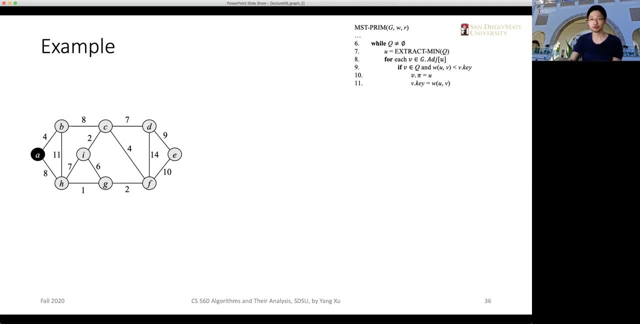 So let's go through the while loop And apparently the vertex a will be the first one being popped out, because it's the root node. right, It's popped out And we need to By the code. right, We need to examine. 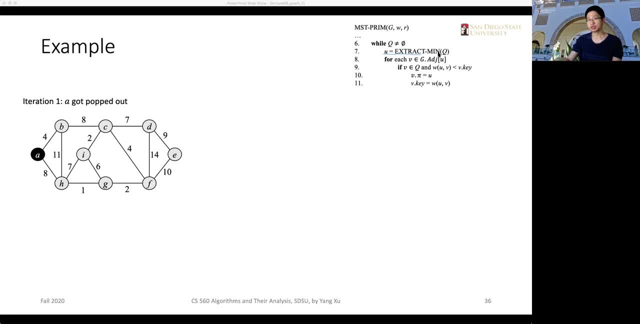 The code says: whenever a node is extracted, we need to go through all of its Adjacent vertices, right? What we have is b and h right. b and h are a's adjacent vertices And they are indeed in the queue because they are all not in the tree yet. 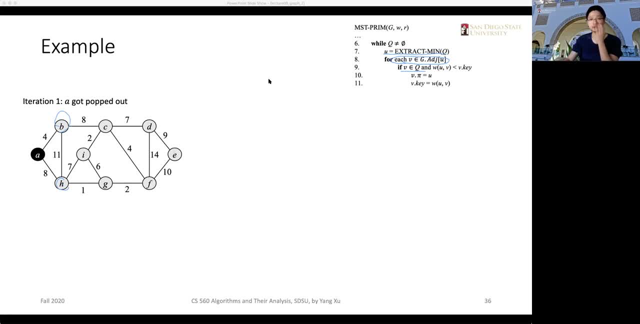 They are all in the gray color, They are in the queue So, And we need to compare their key values with the current weight, with the weight right. We need to compare the weight from u to v with the current key of the. 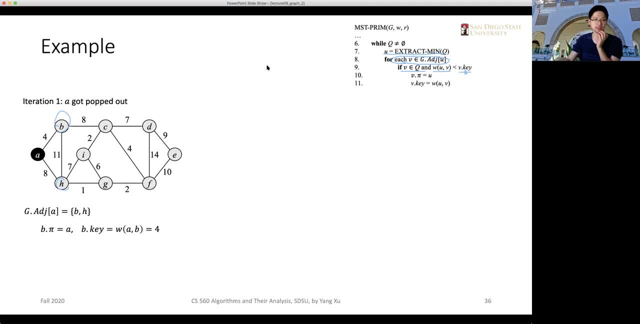 Adjacent vertices. So in this example the parent's attributes of b will be updated to a and the key will be updated to the weights of the ad from a to b right, Because the key is originally infinity and infinity is greater than any number. okay, 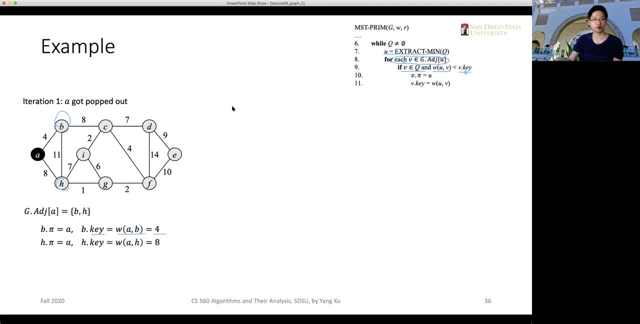 So it becomes four, And same for h. Its pi parent is updated to a and the key is also updated to a And the key is also attributed. So now, after a is popped out, the minimal priority queue is updated. Now we have two non-infinitive 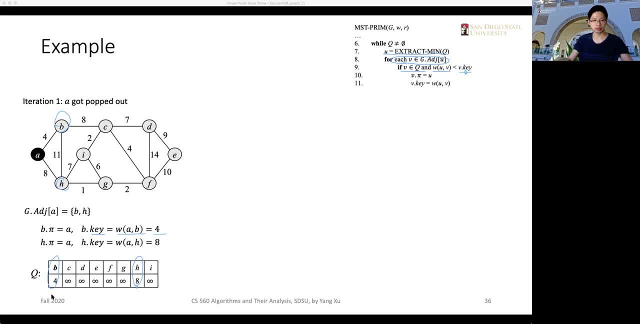 We have two actual numbers. It's for b and h and this is their key values, And the b is highlighted because b has the minimal key value. So b will be the next one being popped out. okay, So in the next iteration of the for loop, 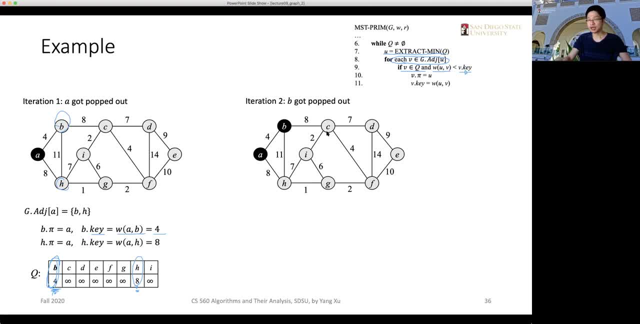 b will be popped out, okay. And after b is popped out, all of b's adjacent vertices will be examined, okay. So after b is popped out because the b's parent is already set to be a in the previous step, okay. 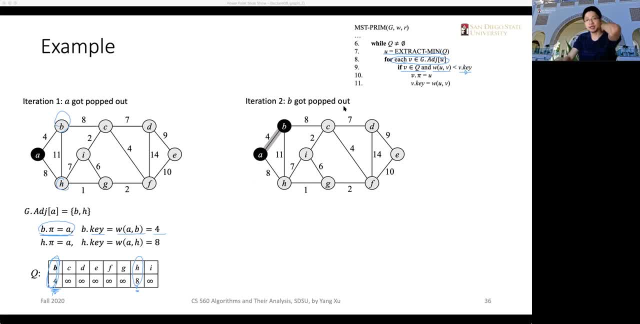 In the previous iteration, The parent of b is a, so we'll have this edge highlighted, indicating the tree path, indicating the tree edge, And a is a root and b is its descendant, is its child. okay, So after b popped out, 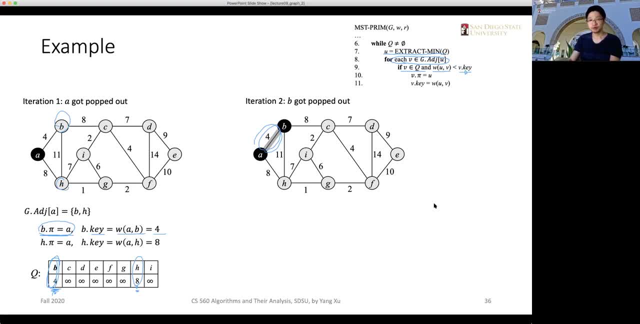 we'll need to check the adjacent vertices of b, which is h and c, and a right a is still its adjacent vertices. But since a is already outside the queue, we don't need to compare the key of a again. We only need to do: 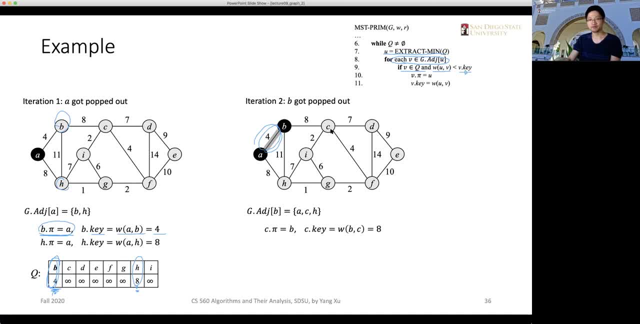 What we need to do is to update the pi parents of b again Of c, by setting the cpi to b and updated the key of c. But we don't need to update the parents of h, Because the key value for h is eight. 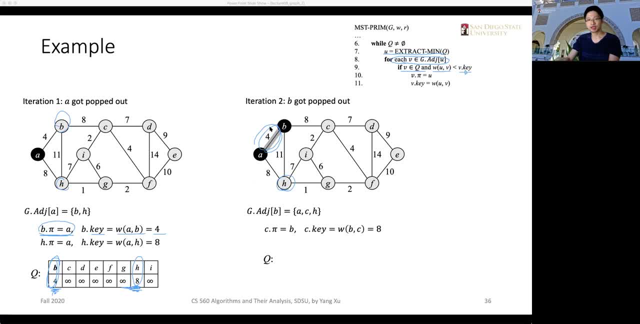 Remember, the old value for h is eight, But the current edge from b to h is 11.. It's bigger than the key, So there's no need to update it. Right, That means the distance from the h to the tree is eight, not 11.. 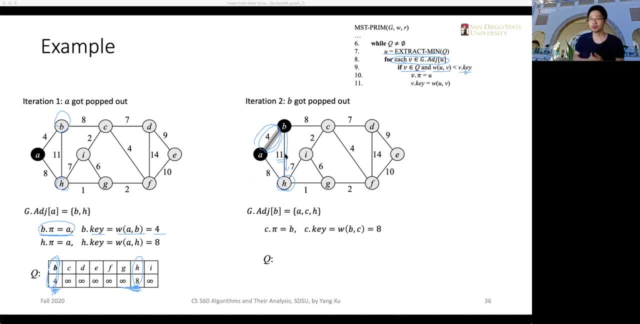 11 is longer, So that's not the actual light weight, right? The light weight is from a to h. Okay, So this step, we don't need to update the values for h. So, as a result, we will have new values in the queue. 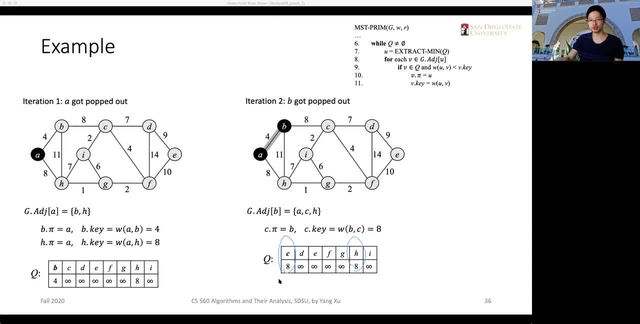 which is c and h. h is not changed but c is changed. Okay, So in the next iteration we have a tie, right, We have c and h And we Basically, we randomly update, We randomly pop out an element from the queue. 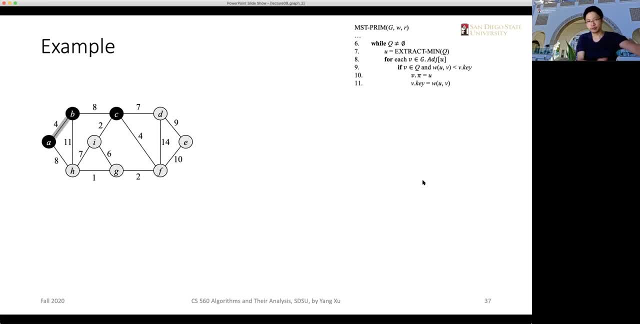 And assume that we pop out c. But it's also possible we can pop out h And the resulting procedure would be a little bit different. But it's okay, It's essentially the same. So c got popped out And we need to check all adjacent vertices. 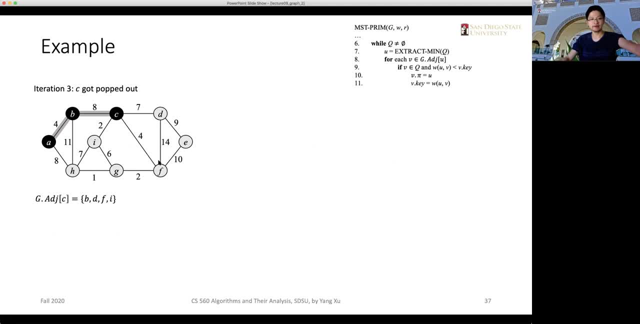 from b i g, From b i f and d right. So accordingly, we need to update the attributes for d, f and i, And b doesn't need to be updated because it's outside the queue. 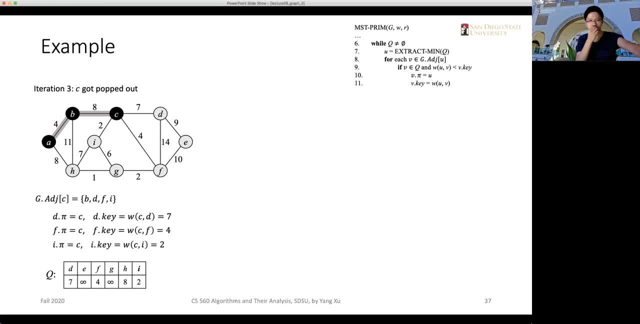 So now the queue looks like this, So the i is highlighted, So the i is closest to the tree And i will be popped out in the next step. Okay, And the i's attribute Adjacent vertices will be checked, which is c, g, h. 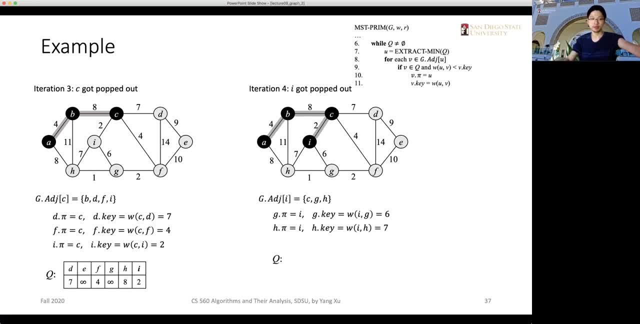 Okay, c, g, h. Now h is updated right. Remember, the old value of h is 8.. But this time the weight from i to h is smaller than h, which means okay, now we need to update your key values. 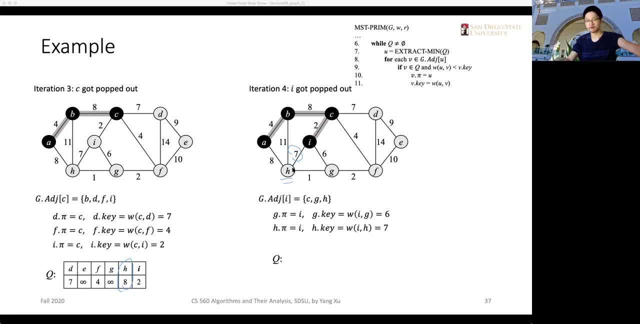 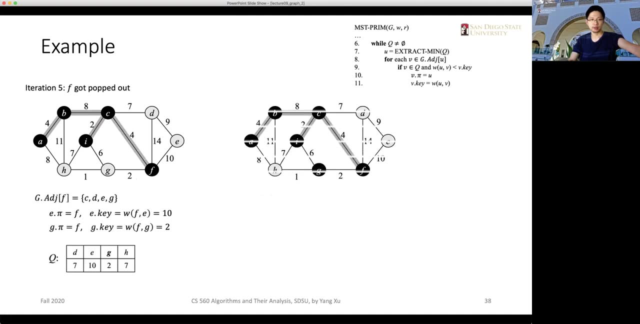 because your shortest distance from h to the tree is now this pass rather than this 8 pass. Okay, So now we need to update it. Okay, So f will be the next one being popped out. Okay, And the queue is updated. 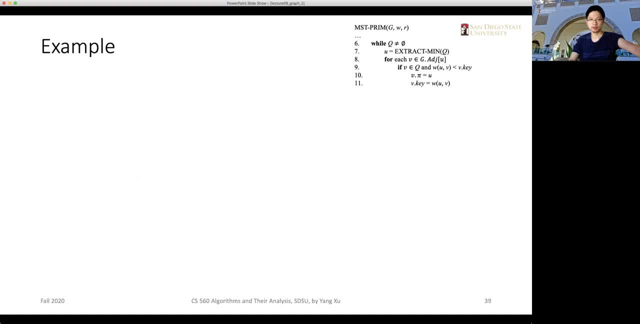 And then g, And then h. Right Now we only have two elements left, So d will be the next one being popped out And e will be the next one being popped out. Okay, And until we reach the empty queue, we will have a complete, minimal spanning tree. 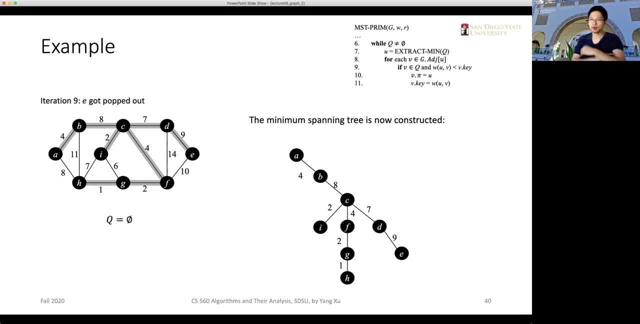 that is constructed now And the tree, all the relationships between the vertices in the tree are indicated by the parent's attributes, the pi attributes. So, starting from the root node, we can able to draw this, We can able to draw the tree structure really quickly. 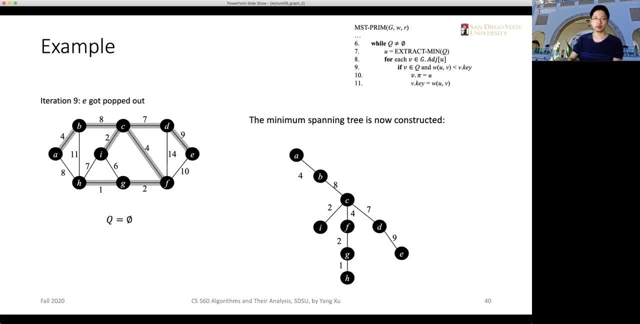 Okay, So that is the Prim's algorithm. So, as you can see, in the process of constructing the minimum spanning tree, we are growing the tree, but we are not merging different parts of the forest Right. The tree is growing incrementally. 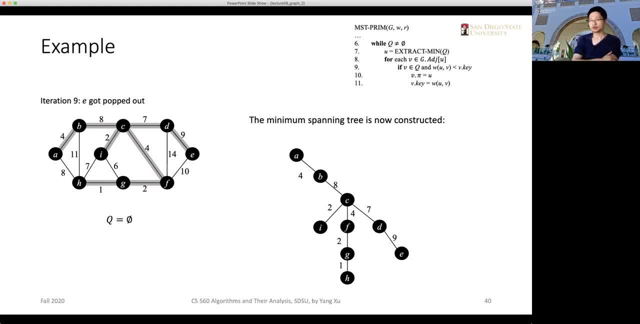 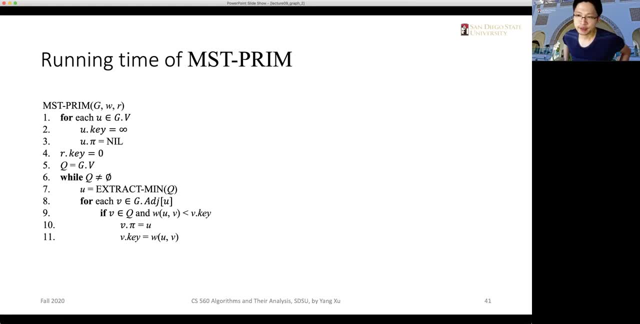 And all the edges in the tree are actually connected, Not separate from each other. All right, So that's the difference, as you can see, from Prim's algorithm to the Carrasco's algorithm. So next let's analyze the running time for MST Prim a little bit. 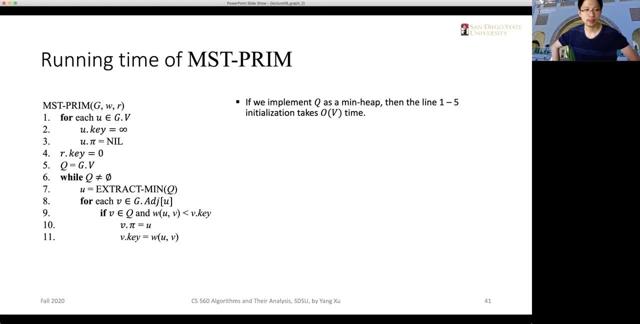 So it's basically the same analysis we need to make. So the initialization takes a big O of V times because we need to go through all the vertices. Okay, And now keep in mind that we have a minimal priority queue maintained and implemented, So the extract mean operation. 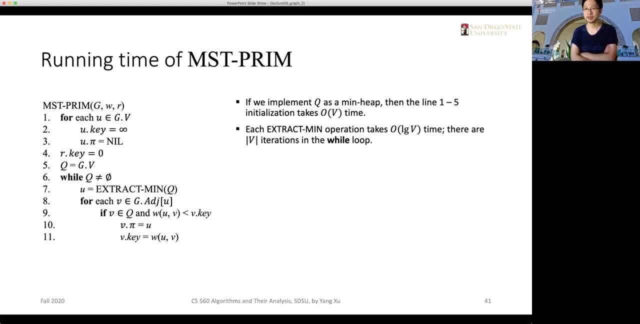 it'll take big O of logarithm of V. So if the, if the the minimal priority queue is implemented by a minimal heap, then because any heap operation is takes logarithm running time, So the extract mean will take take a big O of logarithm V time. 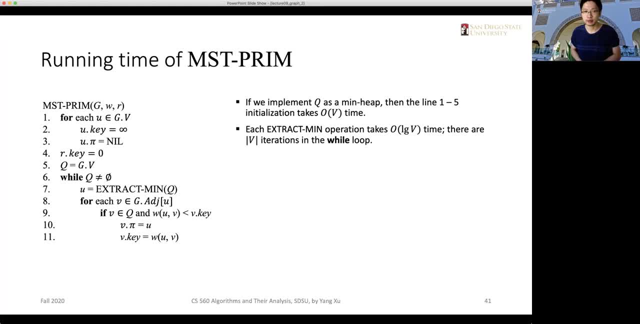 And there's in total V iterations in the while loop, because there's only because all the vertices are in the queue and each, each vertex is it's extracted once. So in total there are V many iterations in the while loop. There are V. 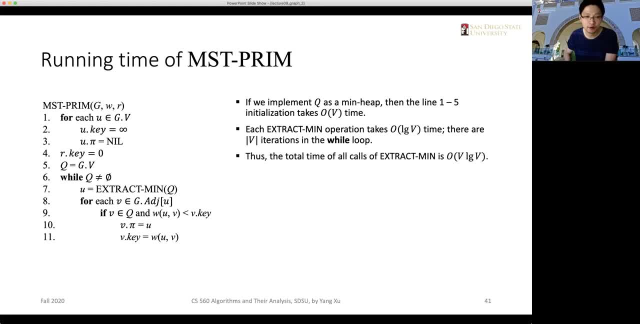 V iterations: Okay, So the total time for calling the extract mean is big O of V times, logarithm of V. Okay, Because it's the extract mean is executed once for each vertex. Okay, And the body from line eight to 11,. 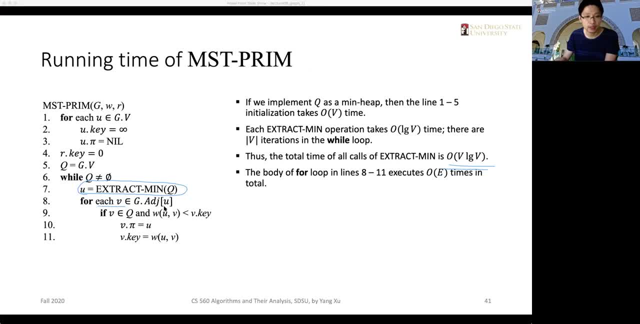 it actually exams all the adjacent vertices for any for for any vertex that is extracted from the queue. So in total we need to consider big O of E times. for all the edges, actually, right, If you go, if you. 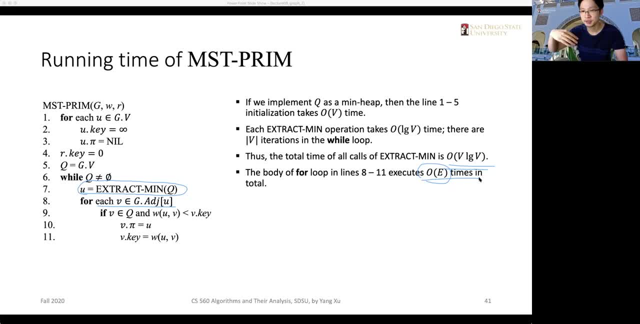 if, for each vertex, you consider all of its adjacent vertices, then actually we're considering all the vertices, all the edges, right? So the body of the for loop executed big O, big O of E times. Okay, Then here comes the tricky parts. 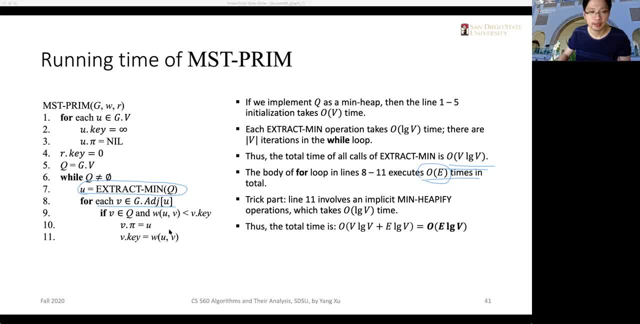 The line 11,. we update the key values right. The key is part of the minimum priority queue. Whenever we update the key value for an element in a queue, the all the elements needs to be rearranged because the key is updated. 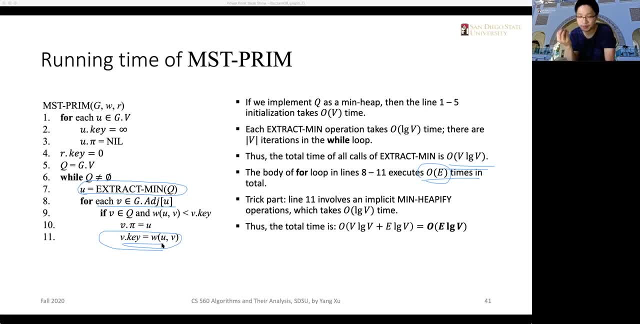 The bigger elements that in the before the updates may may have, may have a higher priority. It needs to be moved into a different position, right? So that's why we each updates of the key will implicitly call the a minimal priority. 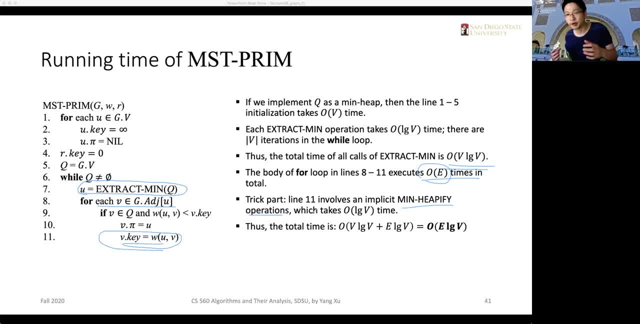 the minimal heapify operation If the minimal priority queue is implemented by a minimal heap. Okay, So that will also cause logarithm of V time each time we update a key. So in total we will have E times logarithm of V associated with this updates. 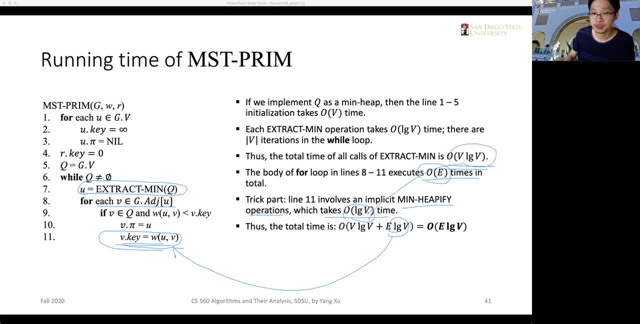 plus the you go V times logarithm of V. here In total we all can. we can have almost a big O of E times logarithm V. So that is the same running time as the cross goals algorithm, which means the prims algorithm is. 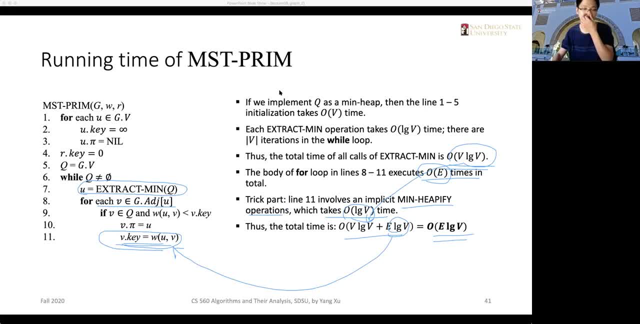 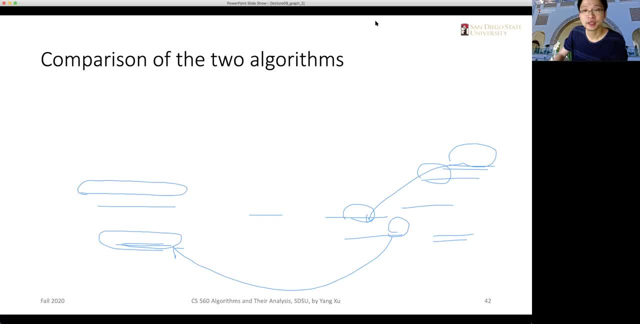 equivalently efficient in terms of running time than the, the cross goals algorithm. But there could be some improvements over the, over the prims algorithm, as we will see later. So let's compare these two elements, two algorithms a little bit. 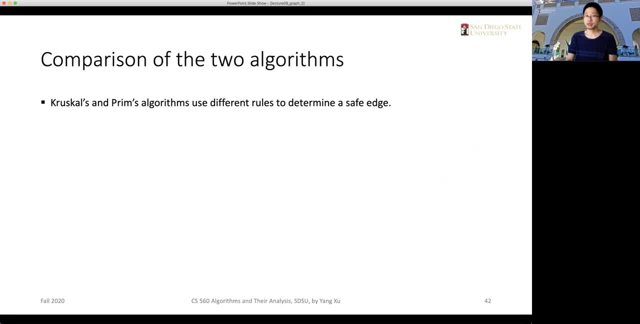 The cross goals algorithm and the prims one. they use different rules to determine the safe edge Right. The safe edge needs to be the light edge, but in cross goals algorithm the light edge is the one with the least weight that connects two distinct 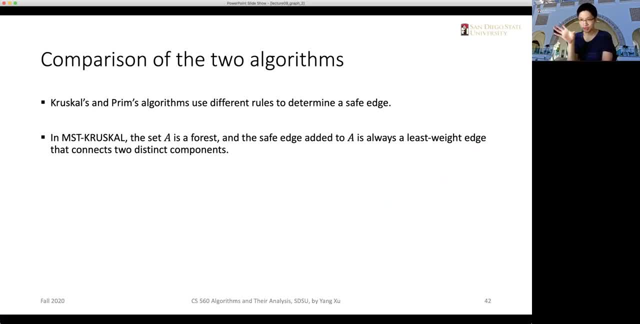 kinetic components or two distinct disjoint sets. So that's the. the weights is is first sorted right First, and then in the while loop, we, you know, in the for loop, we'll go through all the. 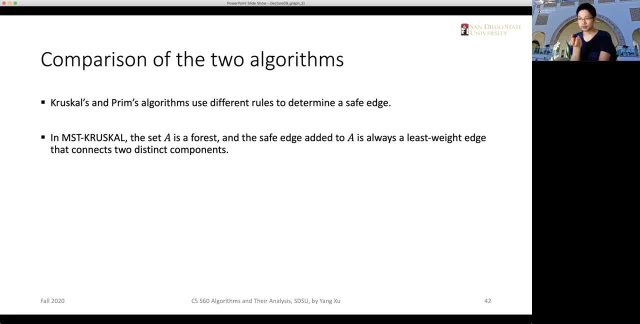 in all the edges in a sorted order, So that's the first one who will satisfy the condition is always the one with the least weight, But in prims algorithm the safe edge is also the one with the least weight, But it's one. 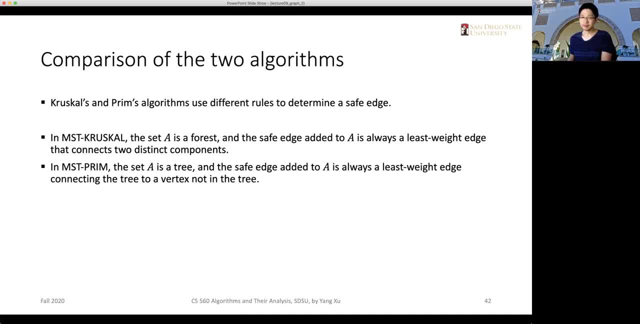 we maintain the minimal priority queue And this least weight edge is connecting a tree to a vertex. They are not connecting two trees. It's not the connection between two disjoint sets or two two trees in a forest, but it's a and a verdict between the 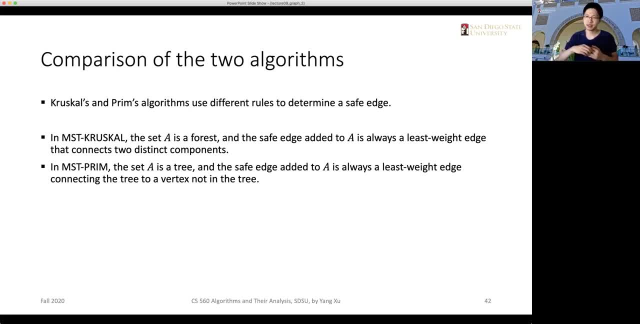 it's the connection between a tree and a verdicts that's outside the tree. Okay, And lastly, let's look at the, the, the, the, the, the and, lastly, the prims algorithm can be faster. 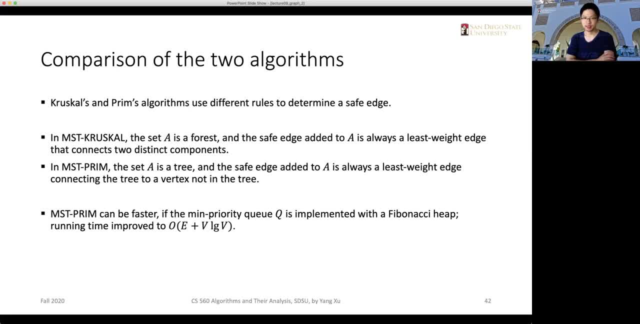 If we implement the minimum prior to queue, we use a more advanced technique like a fibonacci heap. The running time can be further improved by from B, from E times log B to V times log B. Okay, So this is something we 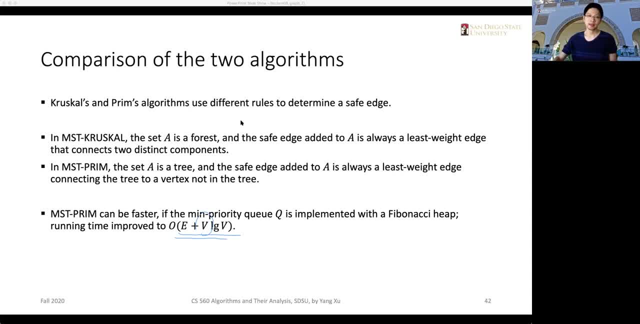 can know about. Okay, Well, And that's basically it for the minimal spanning tree problem. So I think I'm going to end the lecture today a little bit earlier because I think the content so far is a little bit dense, And I hope you can spend more time reviewing the slides and or reading the textbook. 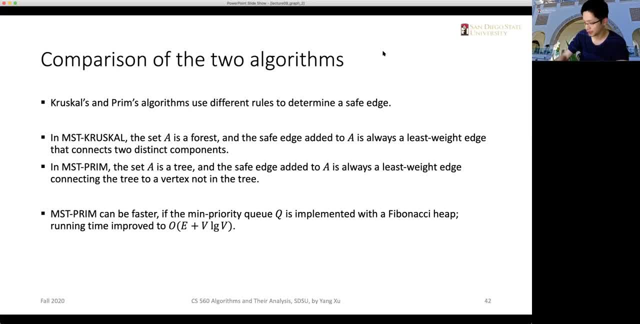 So I will release the quiz questions on the on the campus about the minimum spanning tree problem And also I will release the assignments for release all the questions problem sets for assignments for. So for next week it's Thanksgiving week And but the Tuesday class will still have one class because the school is not closed yet.